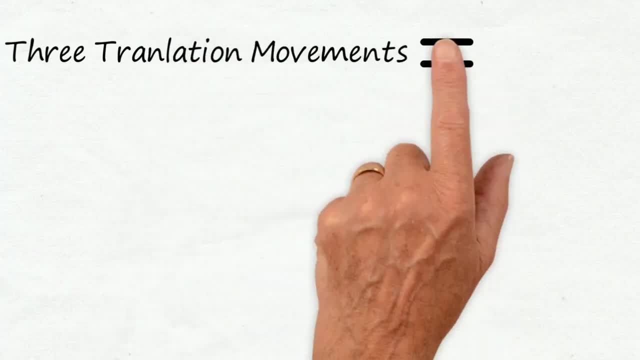 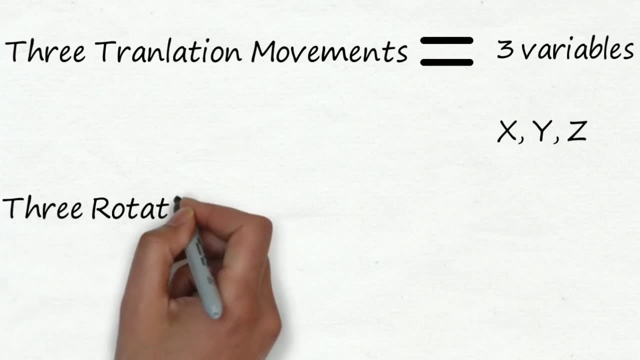 translation movements which can be defined by cartesian coordinates, say x, y and z, And same object has 3 rotation movements. So any object in air has 3 translation movements And same object has 3 rotation movements. And same object has 3 rotation movements. 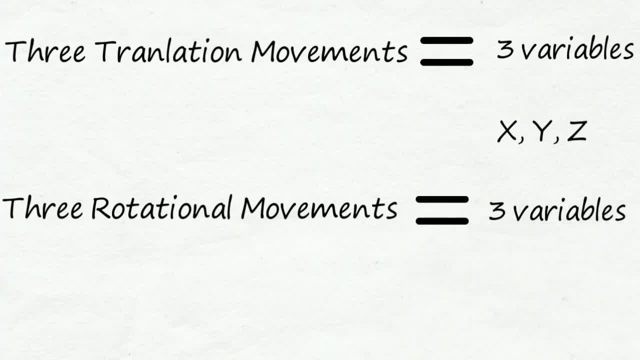 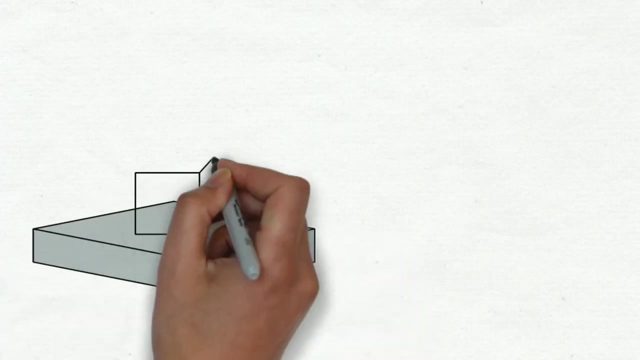 It can also move forward or backward. So these are the rotation movements which can be defined by theta, phi or gamma in polar coordinates. So any object in air has 6 degree of freedom. So these are the movements possible by object which is in air. Now, if box is above this plate, then how much degree of freedom it? 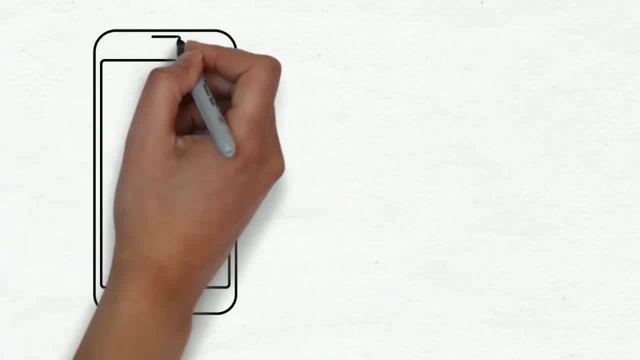 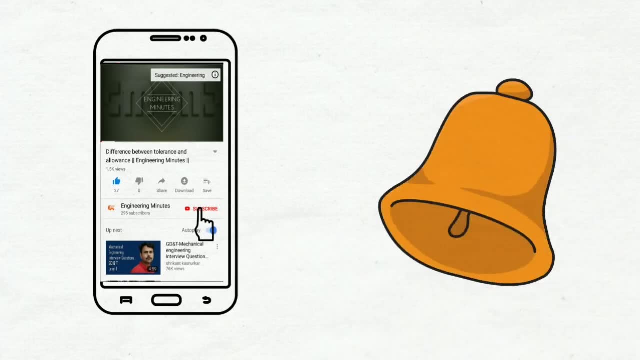 will have. If the box is above this plate, then how much degree of freedom it will have? You can comment it in comment section below. You can also subscribe our channel and press bell icon for regular update. I hope your doubts would be clear by this video. 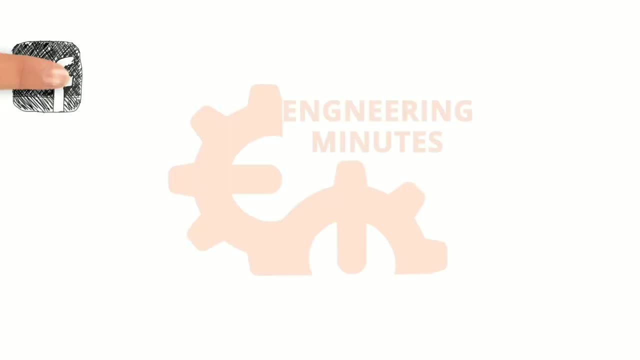 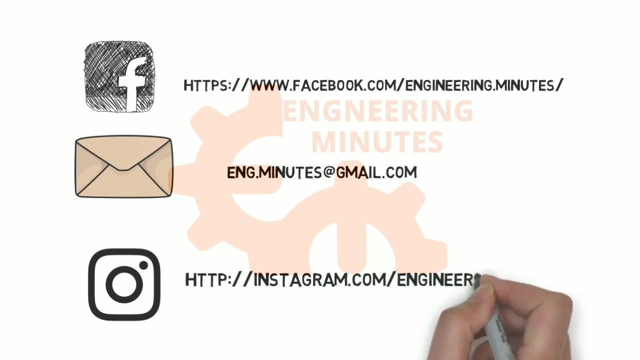 Check out our other engineering videos in engineering playlist. You can like our facebook page, where we put everyday new fact. You can also contact via gmail account. You can also follow our instagram page, on which we put fact everyday. Thank you. 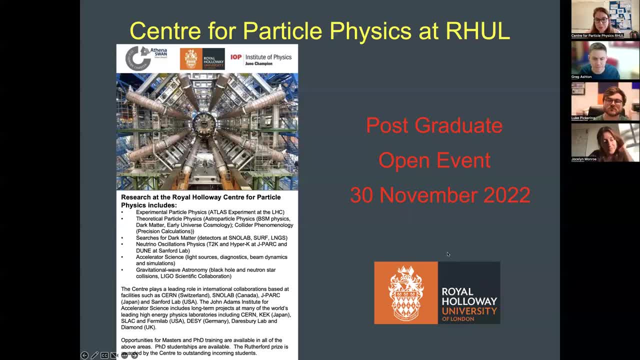 The recording is in progress so hopefully everybody is okay with that. We will be recording the first two parts of this event. So the first part is I will give you some introduction to our center and what are the PhD opportunities. We will also hear from the various research groups. 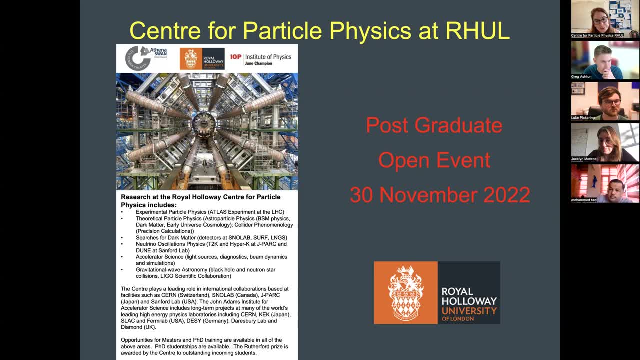 and potential supervisors, academic supervisors in those research groups, And then after that we will have some live tours of some of our facilities here at Royal Holloway, And so after that the final part of this event, around three o'clock or so, will be where we will. 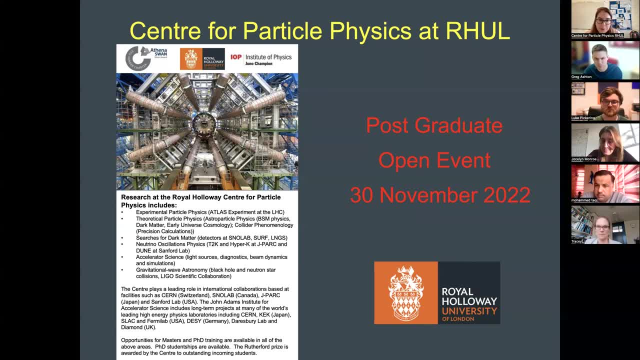 open some breakout rooms in Zoom, And so that will give you an opportunity to go and speak directly to the academics working in the different research group. We will also have a breakout room that will have current PhDs and PhDs in the research group And then after that we will have some live tours.